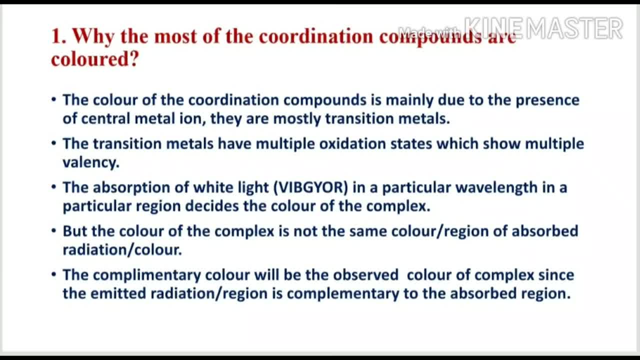 transition metal ions are exhibiting more than one valency, So more than one oxidation state, And it absorbs white light, VIPGR, violet, indigo, blue, green, yellow, orange red. So these are white color, these are white electromagnet radiations. Actually, the metal absorbs the 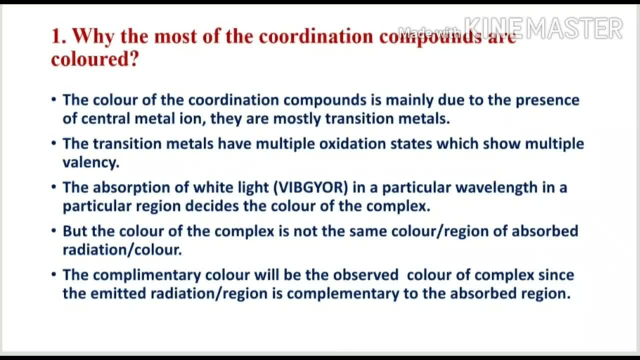 white light and VIPGR in a particular wavelength in a particular region. That decides the color of the complex. But the color of the complex is not the same color or region of the absorbed or color. you see which color or which radiation is absorbed is not the color of that complex. 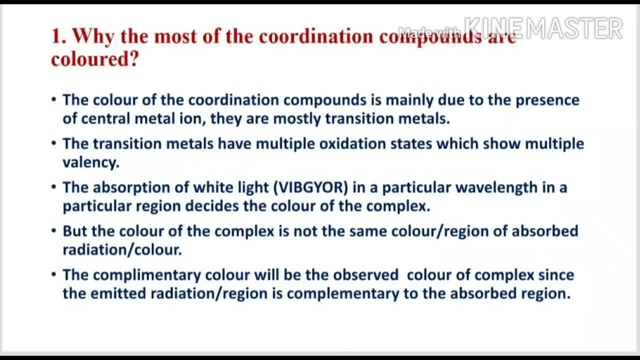 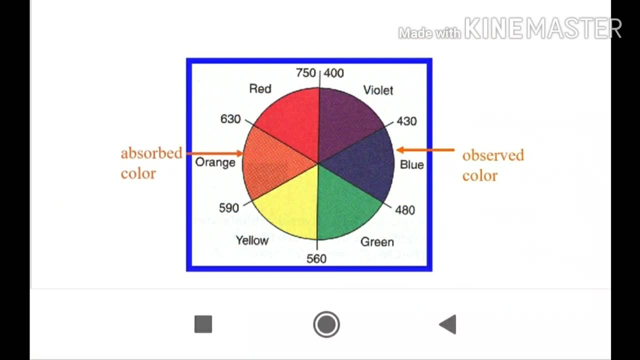 actually the complementary color that will be observed, color of the complex, since the emitted radiation or region is complementary to the absorbed regions. so that is actually very interesting things. we have to notify the color of the complex. so now you see this slide, this artist wheel, this wheel comprises of actually the colors. 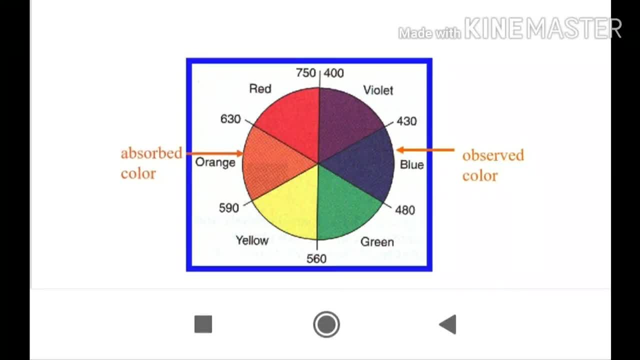 starting from orange, starting from this side: orange, yellow, green, blue, violet and red. so now you see, the left hand side is absorbed color and right hand side is absorbed color. so which color is absorbed? the complementary color, that is, the opposite color, is actually absorbed. for example, if orange radiation is absorbed, 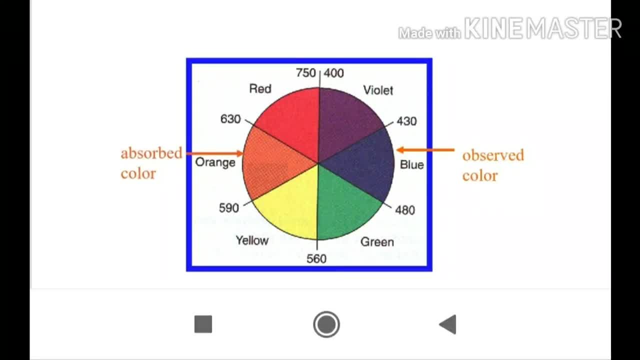 by the transition metal, then the color of the complex will be blue, and vice versa. the same way, if the green color is absorbed by the metal, then the color of the complex will be red. that is the opposite, if sorry. so if the color of the complex is yellow in color, 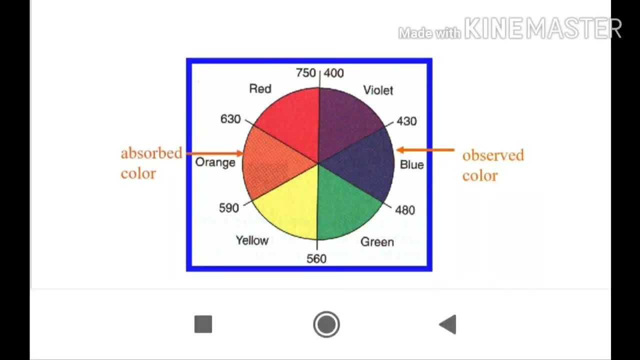 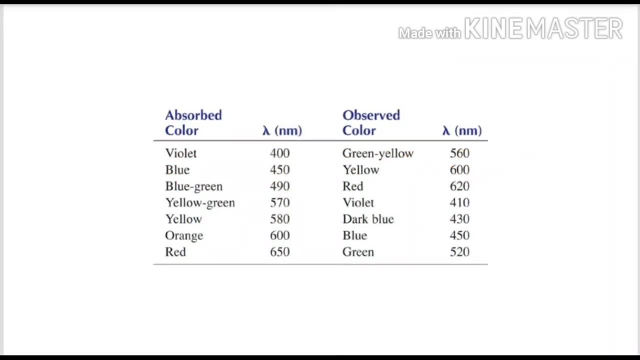 then the violet radiation is absorbed by the metal. so this is the artist wheel. this can easily explain why the color of the complex YAN is different for different complexes. from this slide we can see which color is absorbed and which color is absorbed. for example, you see violet. violet is absorbed at the 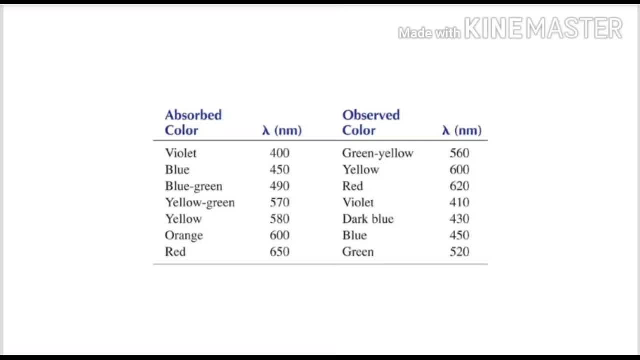 wavelength 400 nanometer, the observed color is green-yellow. in between green and yellow is a mixing of green and yellow, 5-6 nanometer. the lambda is the wavelength. for example, the blue, the absorbed color is 450, and the observed color is yellow, the blue-green. 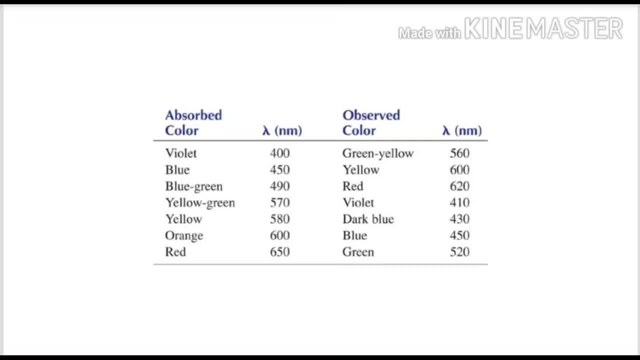 is 490 nanometer and the observed color is red 620 nanometer. likewise the red, the observed at the 620 lambda, that is the nanometer and the observed color is green 520.. so you see, here in this VGR, violet, from violet to red. violet to red, violet is a mixing. 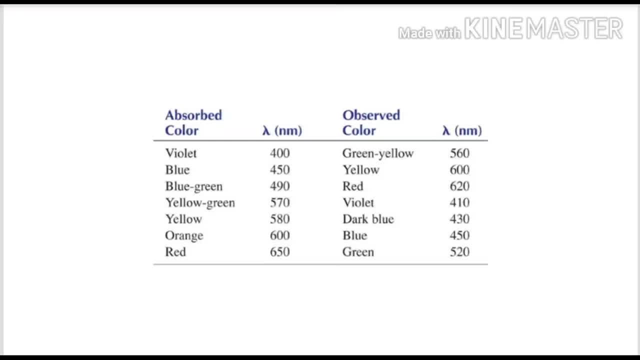 higher energy radiation. red is the lower energy radiation, so the energy wise violet is the violet. to red, the energy is decreased. at the same time, wavelength is increased. that's why the violet has nanometer- 400 nanometer wavelength, whereas red is having 650 nanometer wavelength. but energy is. 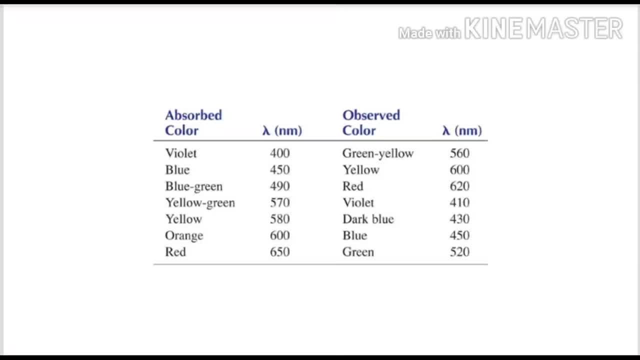 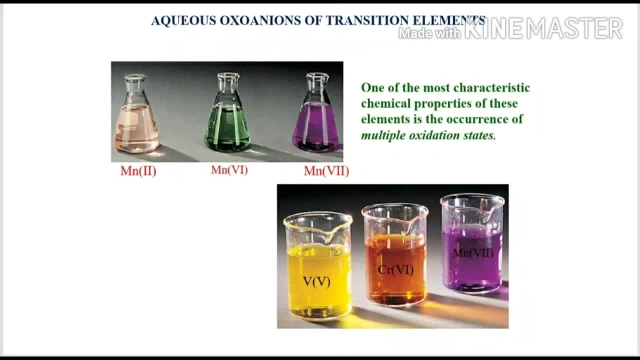 decreased, but the wavelength is increased. one of the most characteristic chemical properties of these elements is a occurrence of multiple oxygen states. already i told. now you see these examples: the manganese 2, manganese 5, manganese 6, manganese 7, so all are manganese, but you see. 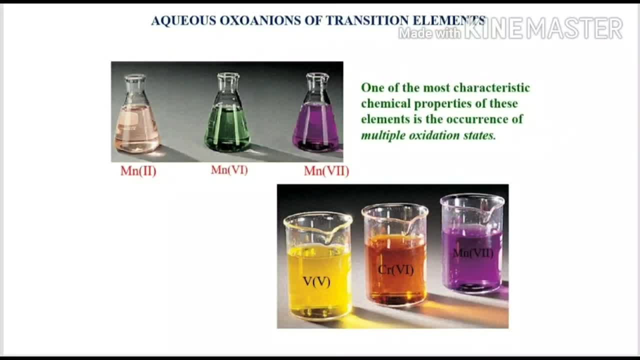 the different colors. the first one is light pink color. second one is a green in color. third one is a deep violet in color. the same way, vanadium 5, chromium 6, manganese 7. so here also you see some different colors. so the color of the complex is mainly due to the, the transition metals. already i told, and this is not. 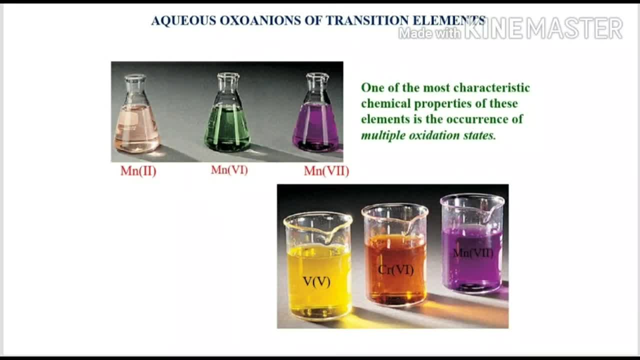 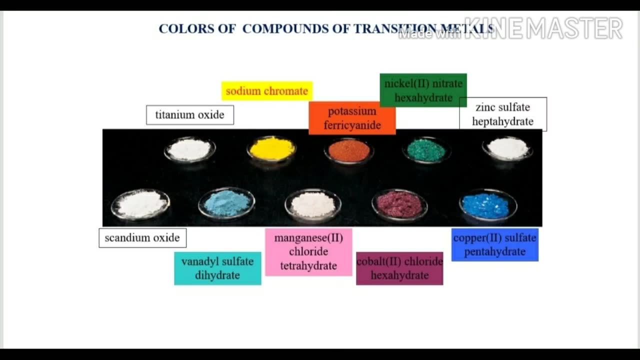 only the color. the transition metals and also the different oxygen states will also give you different colors for the same transition metal. this slide has varieties of the condensation complexes: チ adalahơn sulfate diatate- light blue in color. scandium oxide is a white in color. so because all these 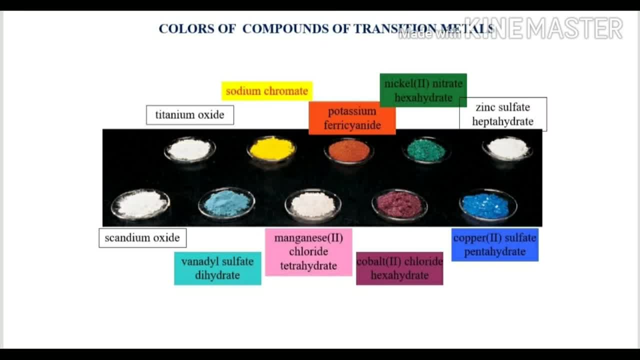 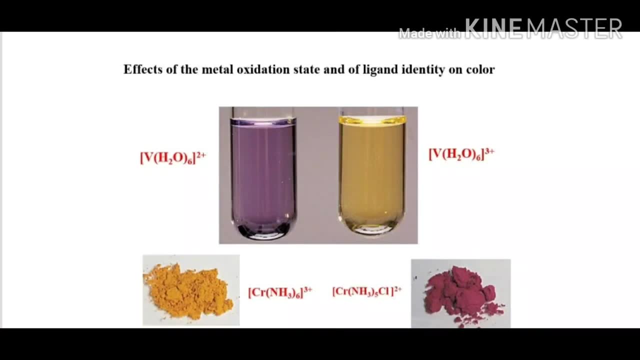 colors. that is a difference. also showing the different colors. the main reason is the metal. so this metal, the absorption of metal, are to be for particular wavelength or region. that will decide actually the color of the complex. the oxygen state influences the color of the transition metals. how transit is a. 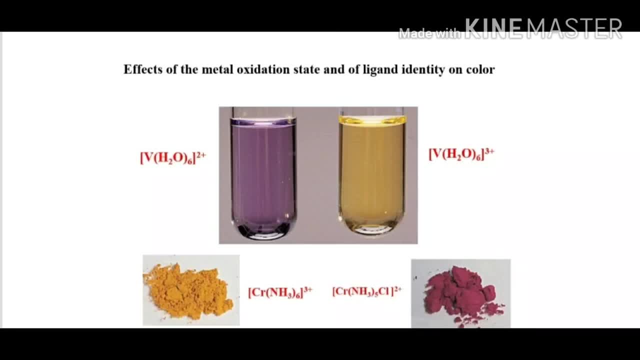 coordination complexes. you see, the first one is the hexa aqua- vanadium 2 ion and the second one is hexa aqua- vanadium 3 ion. both are somewhat at same type of complex, but the only difference is in the oxidation stage. the first one is oxygen state is two, the second one is oxygen is three. 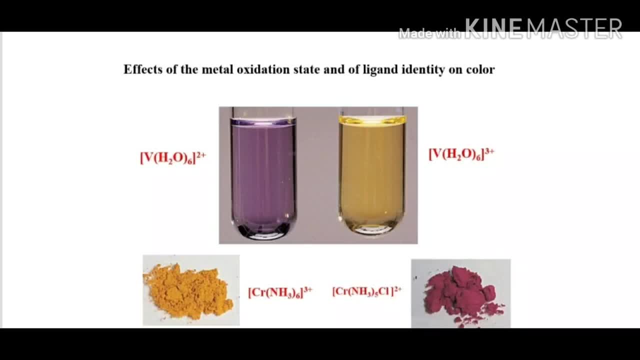 but it shows different colors. the first one is somewhat is a light violet in color. the second one is somewhat yellow in color. the same way. the another example: examine chromium 3 ion and exam a pentamine chloro, chromium 2, iron. so both has chromium as a central metal ion, but the first one 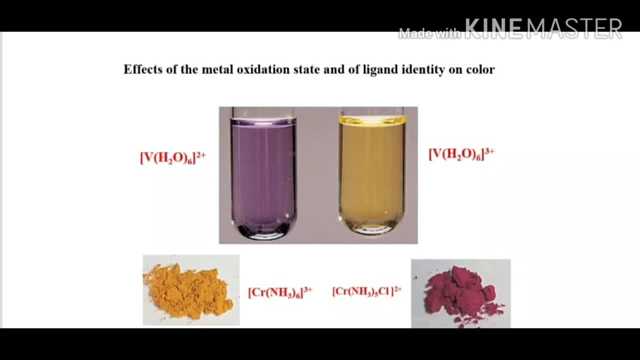 has. all six elegans are same. the second one instead of one. i mean ligand, chloro ligand is substituted. so because of this substitution, what is the difference? you make the very, very visible difference between these two counters. the first two, one is somewhat yellow in color, the second one is somewhat red in color. so if you substitute, if you replace one of 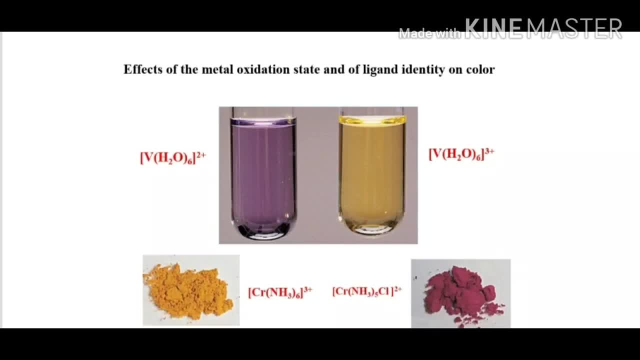 you replace one ligand and substitute by another ligand, that will give you a different color. so so the color of the complex is mainly due to the central metal ion and, in other way, not only the central metal ion plays a main, important role in the color of the canvas, as well as oxygen state. 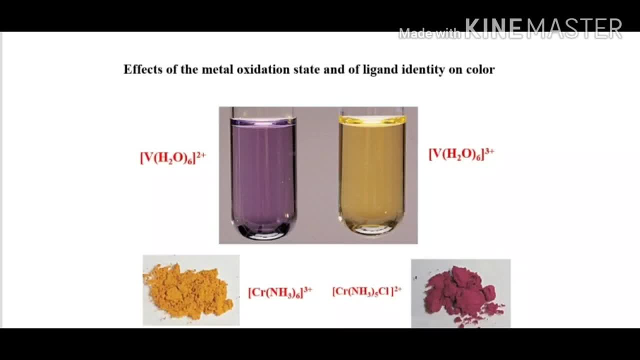 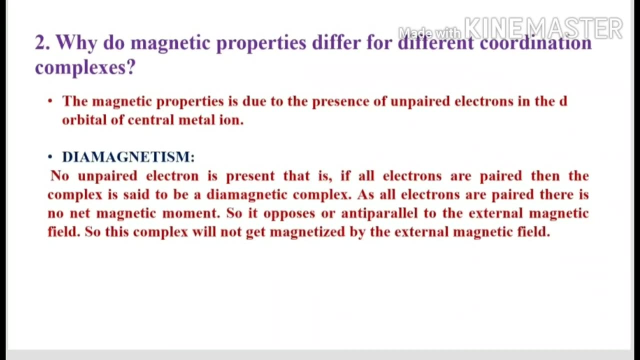 and also the ligand. so all are very important for the characteristic color of the coordination complexes. the second title of this is magnetic properties. why do magnetic properties differ for different coordination complexes? that's also very, very important one in the coordination chemistry. the magnetic properties is due to the presence of unpaired electrons in the d orbital of central metal ion. 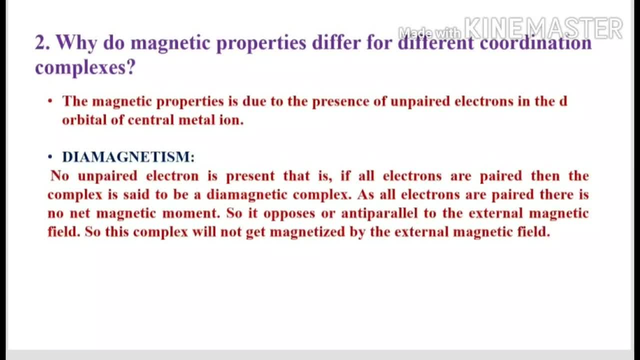 what is meant by unpaired electron. you see, every orbital has maximum two electrons. if there are two electrons present in an orbital, both are having opposite spin. one is spinning in the clockwise direction and the other is spinning in the opposite direction. so the two electrons are present in the anti-clockwise direction. another electron will be spinning in the anti-clockwise 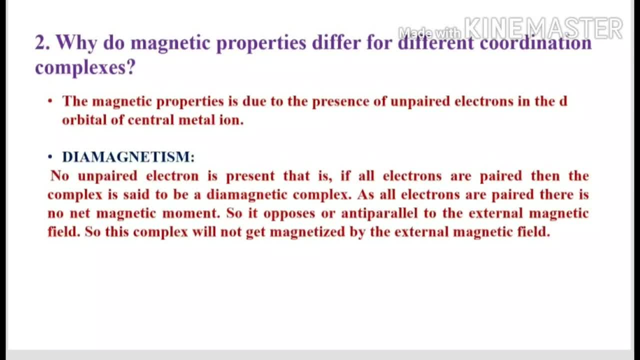 direction. so when two electrons are present the spin will be different. it is opposite. so this is known as the paired electrons. but if only one electron is present in one orbital- for example, you see the p orbital- there are three p orbital that are px, py, pz, totally three orbitals. so 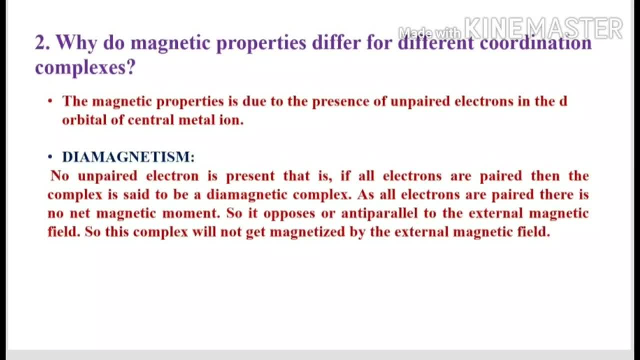 maximum six electrons may be present, can be present in the p orbitals, but all. if all six electrons are present, then all are paired. so if all six electrons are present, then all are paired. but if only five electrons are present, then the third orbital will having will have only one. 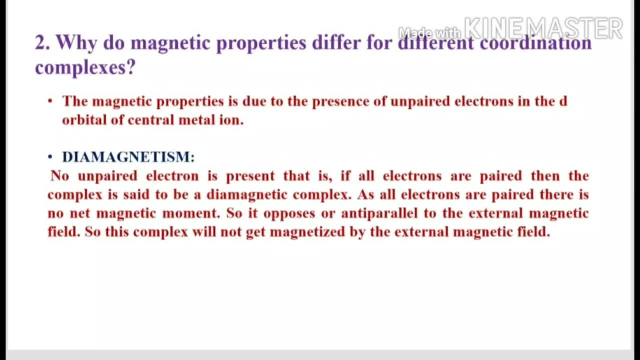 electron. now it is an unpaired electron. so if only one electron is present in an orbital, that electron is not unpaired electron. so minimum one unpaired electron and more than one unpaired electron may be present in orbitals that will decide the magnetic properties of the complex. so the 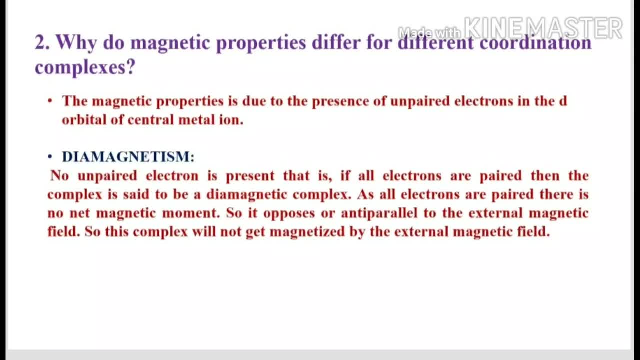 magnetism or different types of magnetisms are there? diamagnetism, paramagnetism, ferromagnetism, ferrimagnetism. many different mechanisms are there. first one is a diamagnetism. what is meant by diamagnetism? no unpaired electron is present. that is, if all electrons are paired, then the 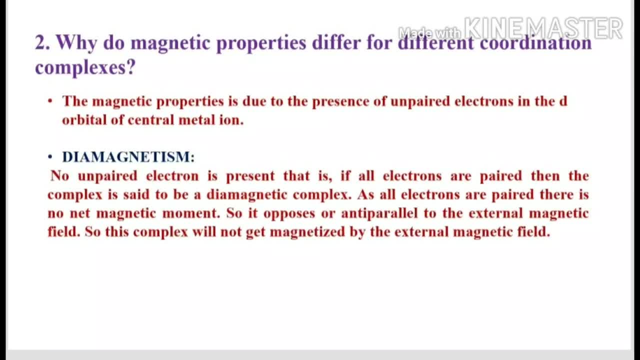 complex is said to be diamagnetic complex, as all electrons are paired. there is no net magnetic moment. actually the magnetic the field is given by the unit magnetic moment. that means the magnetic field that is given by the unit magnetic moment. so it opposes. there is a diagram, if the diagram 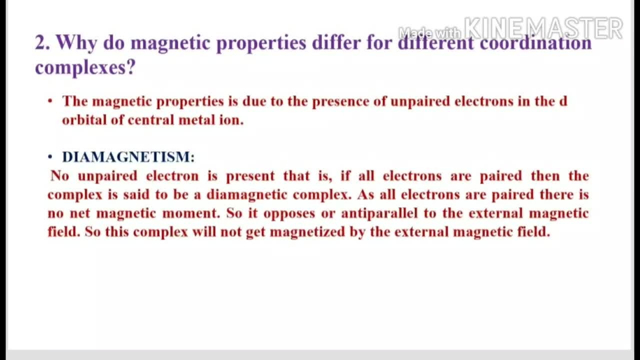 it is, all electrons are paired, then there is no net magnetic moment. so it opposes or anti-parallel to the external magnetic field. if you apply the external magnetic field from outside to a complex, that that metal, actually that metal. if it is that metal they are hanging the paired electrons into. 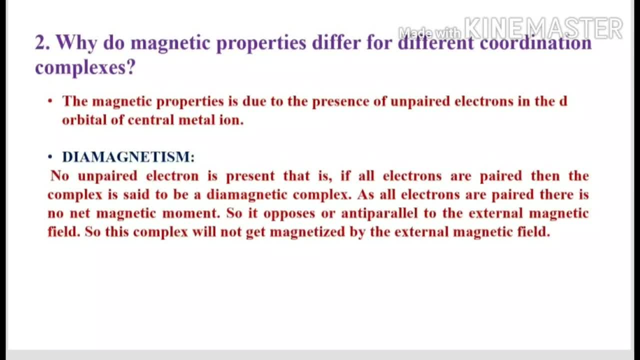 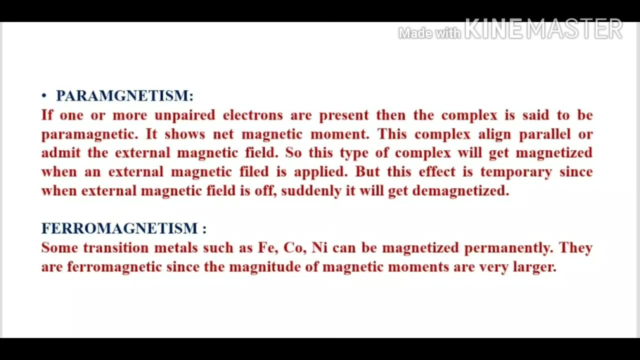 orbital, then what will happen? the external magnetic field will be opposed by the these diamagnetic properties of this complex. so this complex will not get magnetized by the external magnetic field. the next one is paramagnetism. if one or more unpaired electrons are present, then the complex. 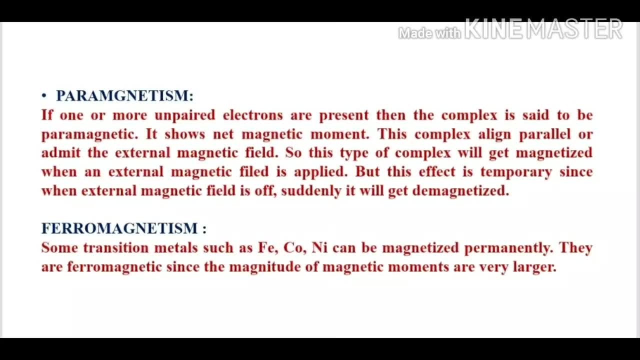 is said to be paramagnetic. it shows net magnetic moment. this complex align parallel or admit the external magnetic field. so this type of complex will get magnetized when an external magnetic field is applied. but this effect is temporary since when external magnetic field is off, suddenly it will get demagnetized. so this is the magnetic moment. value is: 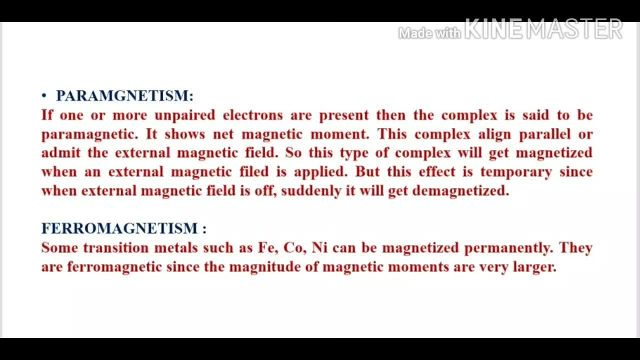 very small for this paramagnetism. the next one is ferromagnetism. some transition metals, such as iron, cobalt, nickel, can be magnetized permanently. they are ferromagnetic since the magnitude of the magnetic moments are very larger. in this slide, the following exam will show the magnetic properties. 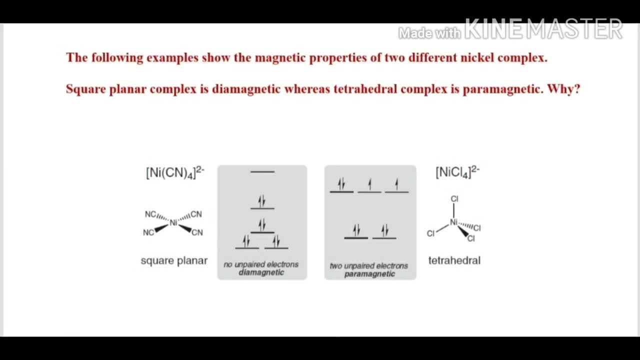 of two different nickel complex. square planar complex is diamagnetic, whereas tetrahedral convex is paramagnetic. two different complex i have given in this slide: tetra sino nickelate two ion. the first one is square planar, the second one is tetra chloro nickelate two ion tetragattal. 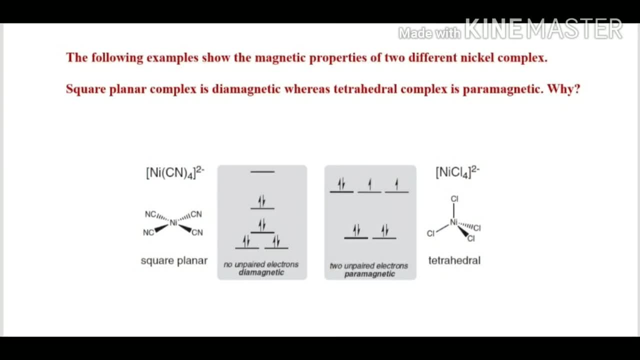 both are nickel convex, but the ligand is different. here the cyano ligands are present, here the chloro ligands are present. the first one is square planar, the second one is tetragattal. the very interestingly, both are having the same coordination number. 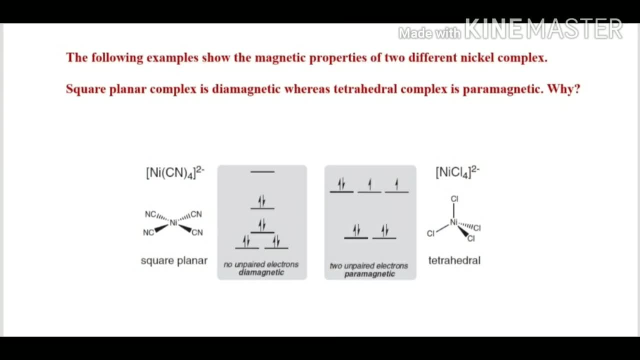 same coordination number and the same oxidation number, but the structure is different. the first one is a square planar, second one is a tetrahedral. but you see, very interestingly, you see, the first one is a diamagnetic, second one is a paramagnetic. the reason is because 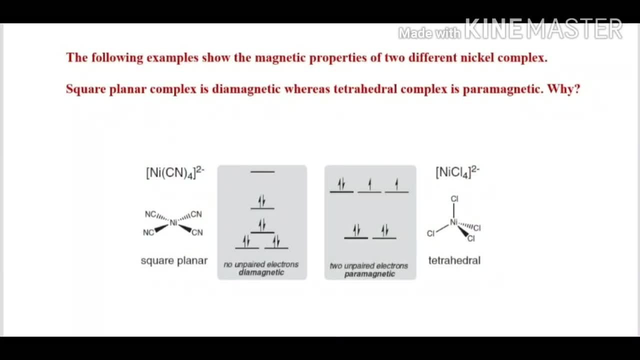 in this orbital all electrons are paired for the square planar complex, but in the tetrahedral complex there is two unpaired electrons are present, so it is a paramagnetic. so what is the reason for that? why? first one is diamagnetic, second one is a paramagnetic. first one is: